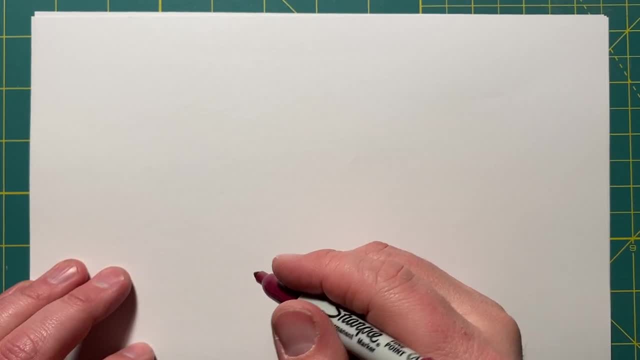 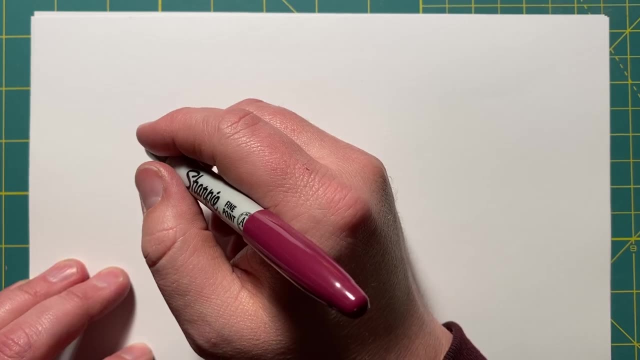 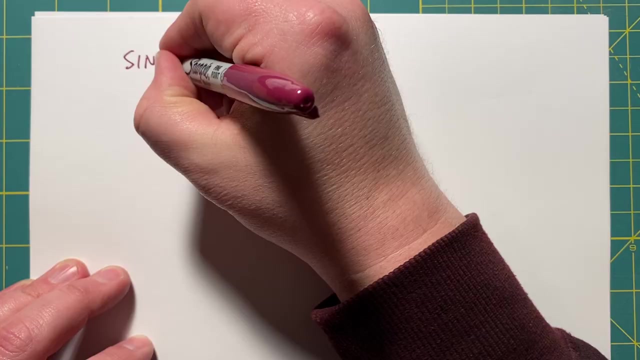 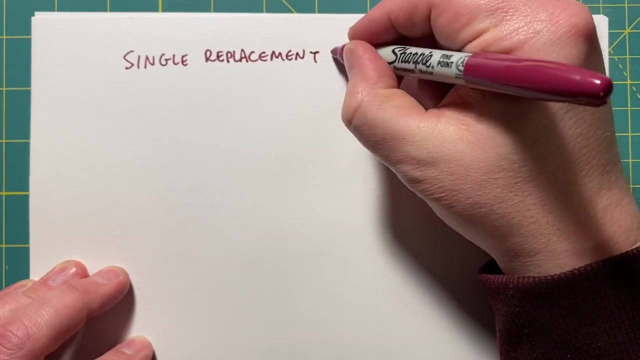 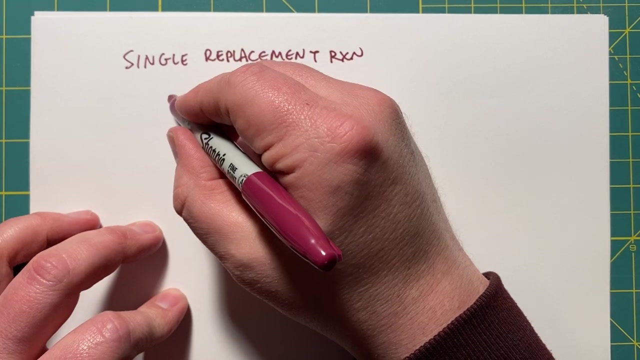 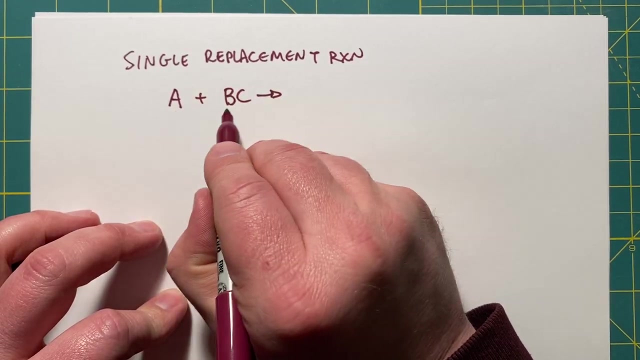 Welcome to Chemistry Tutorials with Cabbage. Today I'm talking about different reaction types. I'd like to show you how to do the single replacement reaction- It's also called single displacement. In this one. this is a single replacement reaction, The basic form. it could have two different forms. One of them could be where we have something like this and we end up with the A displacing the B, So we end up with AC plus B. 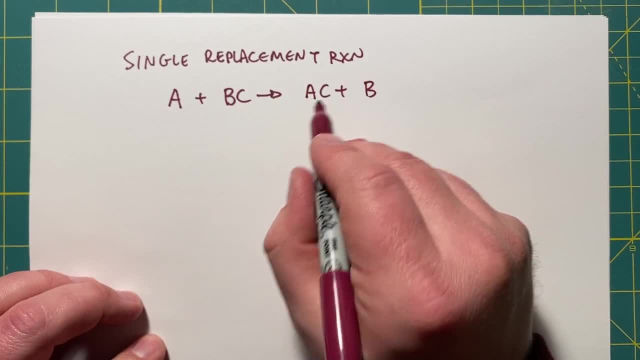 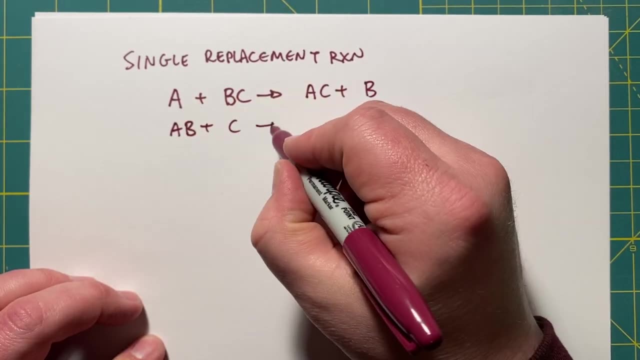 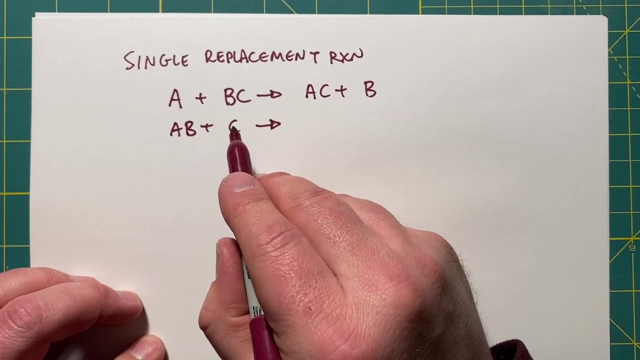 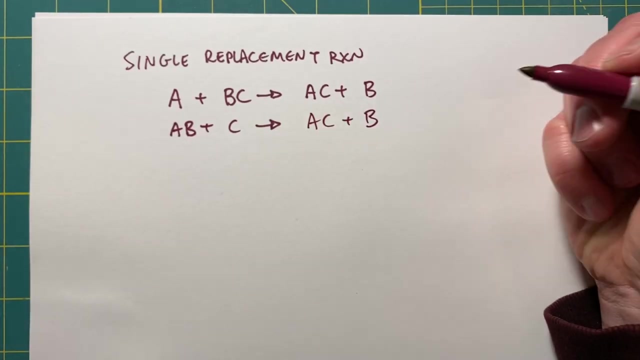 Alternatively, we may have something displacing something else, and so it might look a little different, but we should recognize both of those, So we might have something like AB plus C. It doesn't have to be in this order, of course, but we end up with: in this example, the C would displace the B, and so we end up with AC plus B. 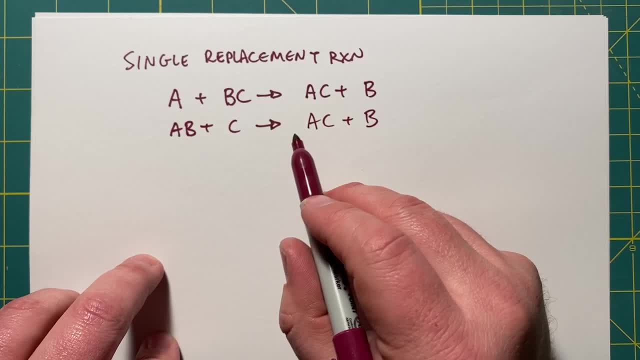 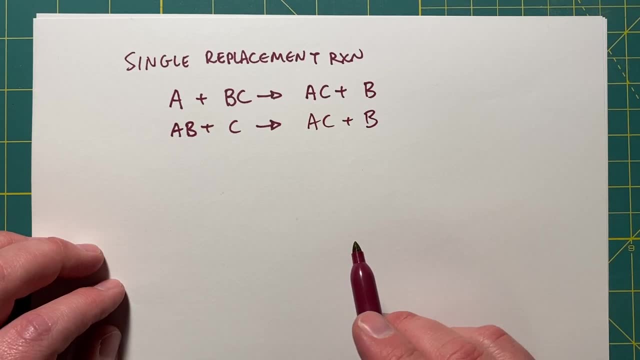 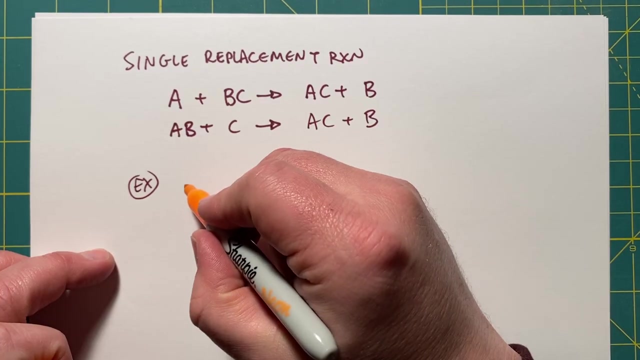 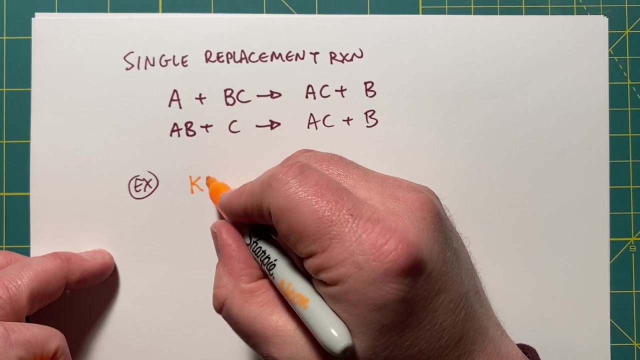 I know that the result looks similar. It's because it's a single replacement, but what it's replacing is a little different. Let's look at one such example. Alright, one such example, One such example that we might see in a lab is where let's say we have a reaction, where let's say about potassium bromide and we're going to react it with, say, fluorine gas. 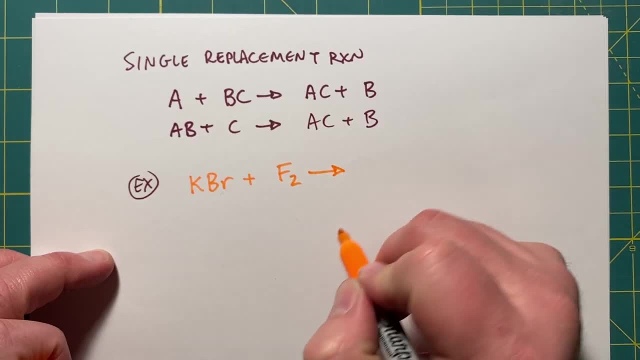 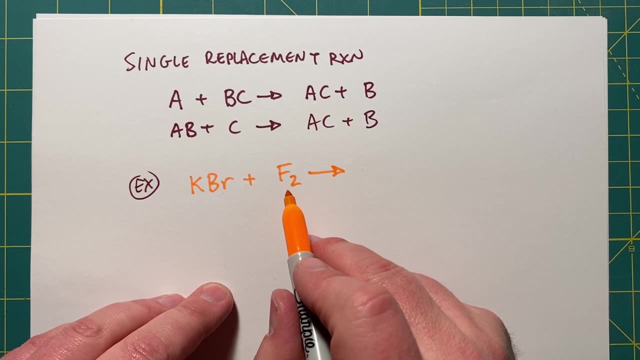 We wouldn't do this in the lab. That would be dangerous. But what's going to happen is, in this example, the fluorine which forms an anion is going to be negatively charged and it's going to displace the other negatively charged thing. 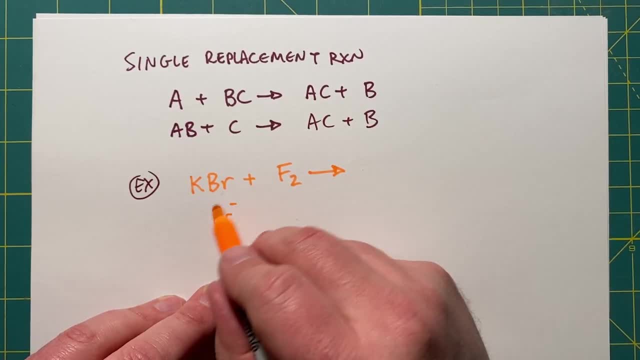 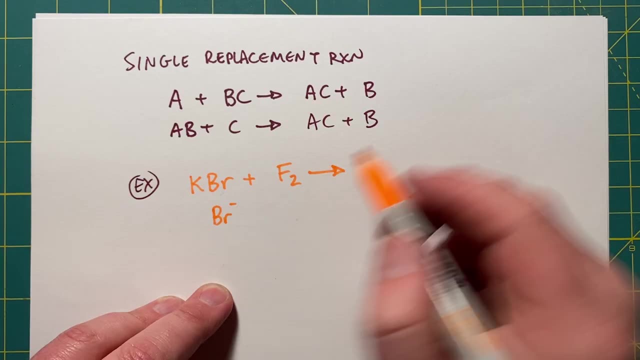 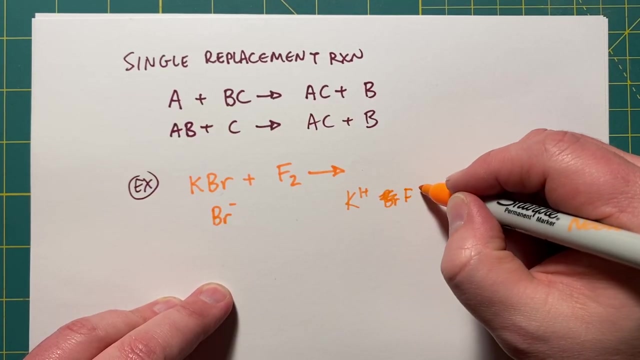 So bromide- here this is potassium bromide- is Br negative and this fluorine, as it combines with the metal, forms an ionic compound and it's going to make potassium fluoride. Potassium is a 1 plus. Bromide as an fluoride, as an anion, is a 1 minus.